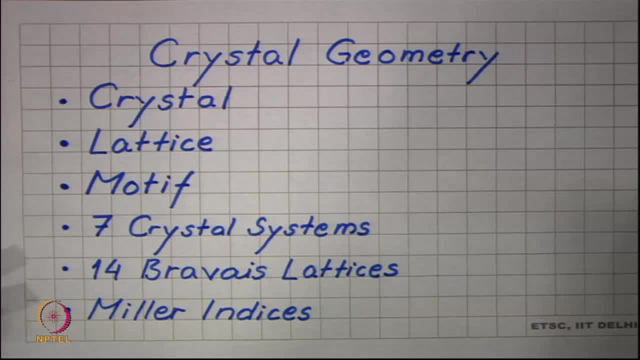 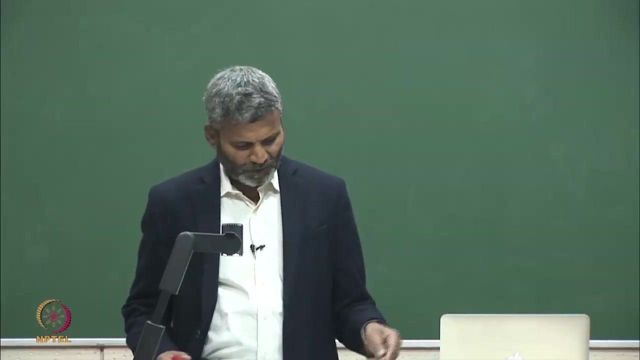 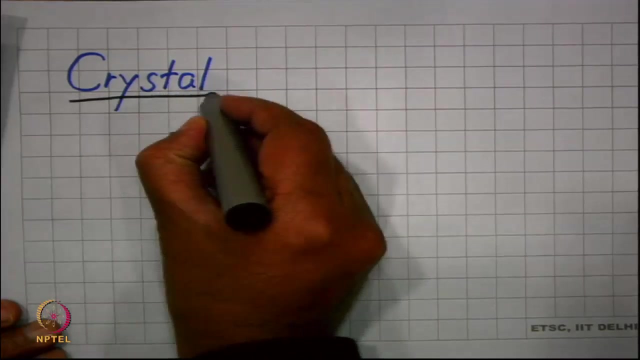 and see how the lattices can be classified into seven crystal systems and 14 Brevet lattices, And we will end this section with discussion of Miller indices of directions and planes. We begin with the definition of crystal. What is a crystal? So you can pause here. 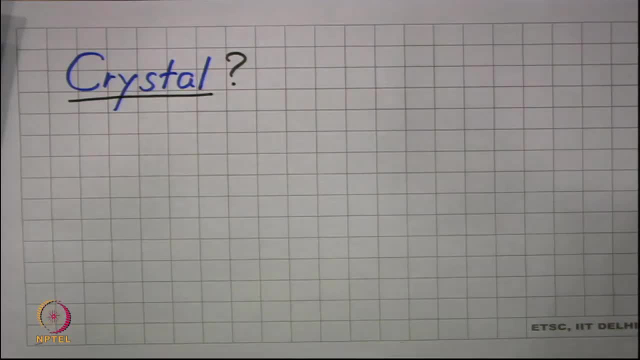 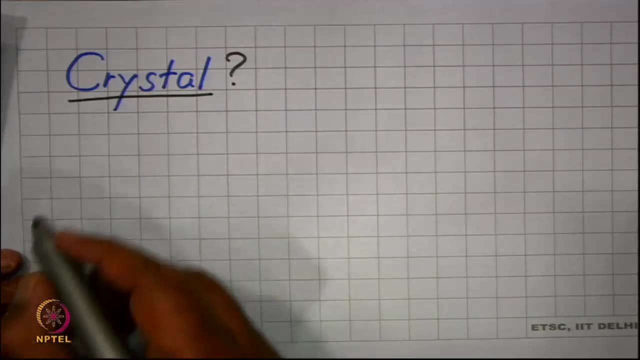 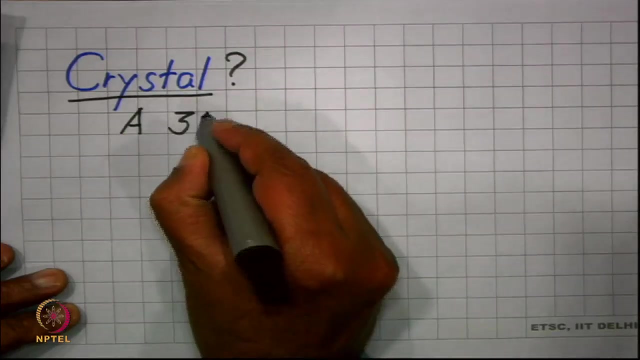 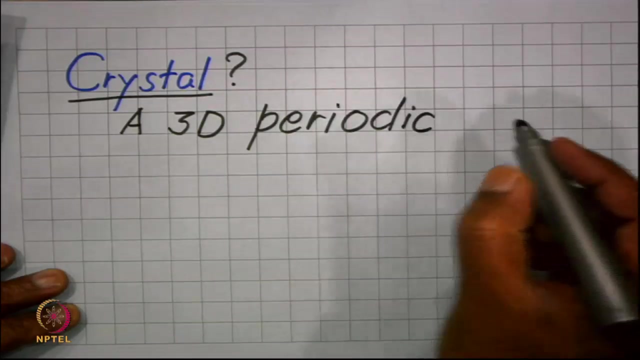 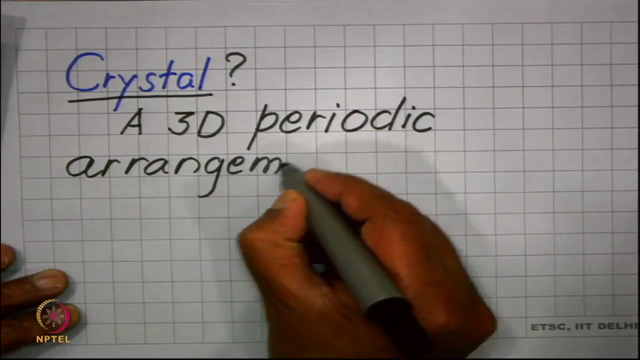 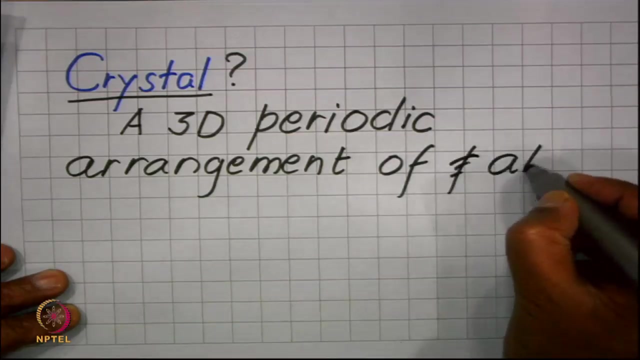 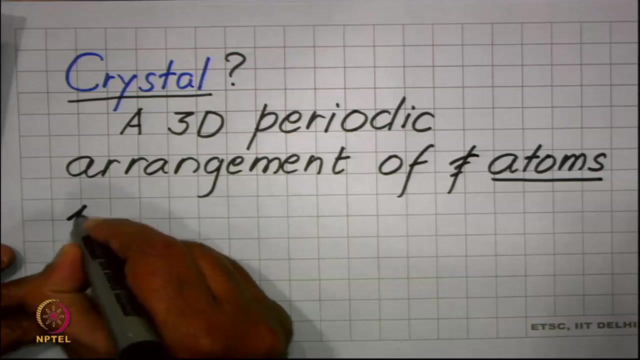 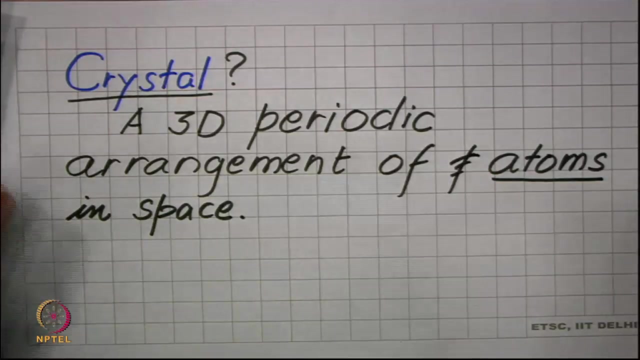 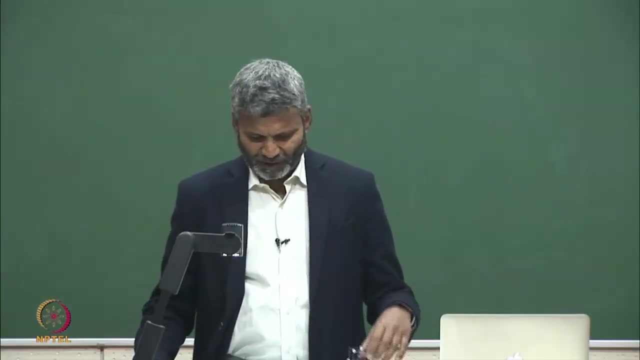 And think about what is your definition or what is your concept of crystal before I give my definition. We will define crystal as a three-dimensional periodic, non-linear arrangement of points or, sorry, of atoms. A three-dimensional periodic arrangement of atoms in a space will be called crystal, The related concept. let me show first a 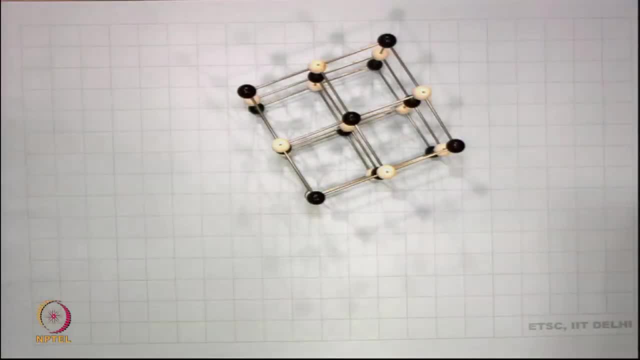 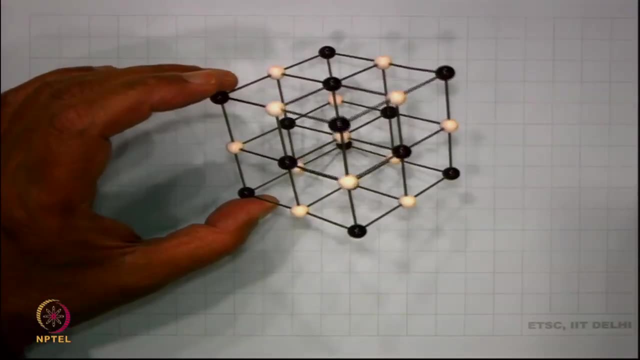 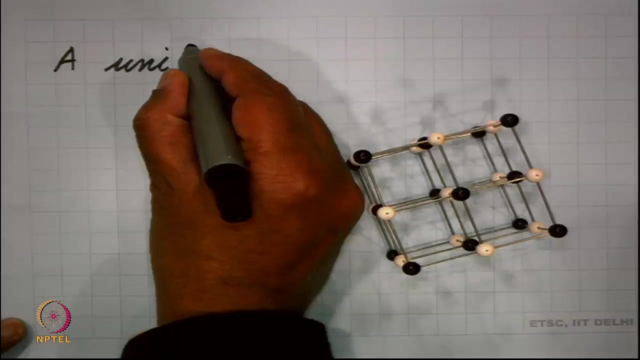 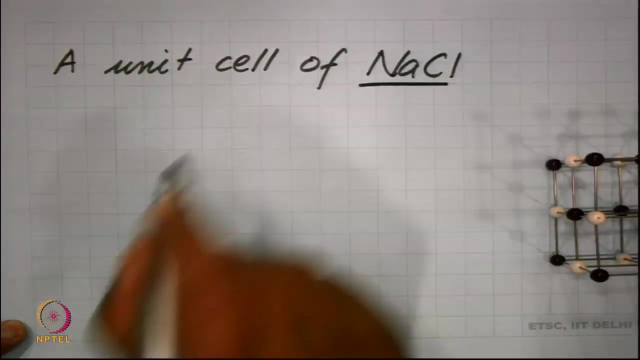 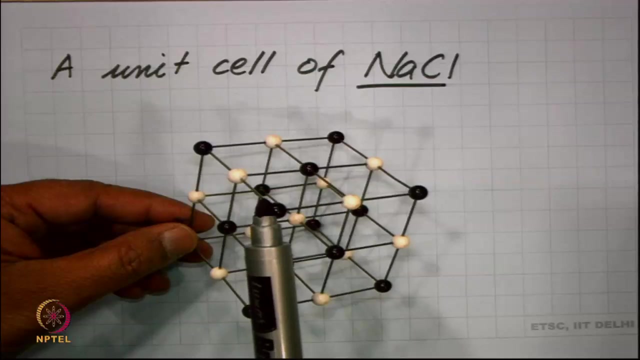 model. This is a model of what we mean by three-dimensional periodic arrangement of atoms. So here is a unit cell of sodium chloride. So this is unit cell of sodium chloride. The black atoms you can consider as chlorine, the white ones as sodium, And what we mean by three-dimensional 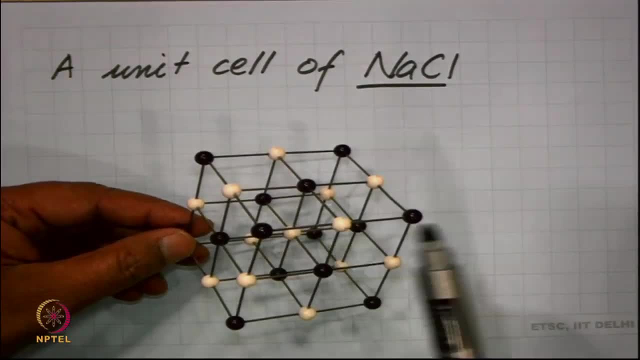 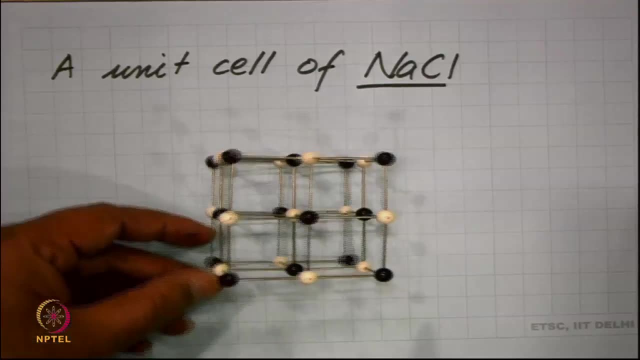 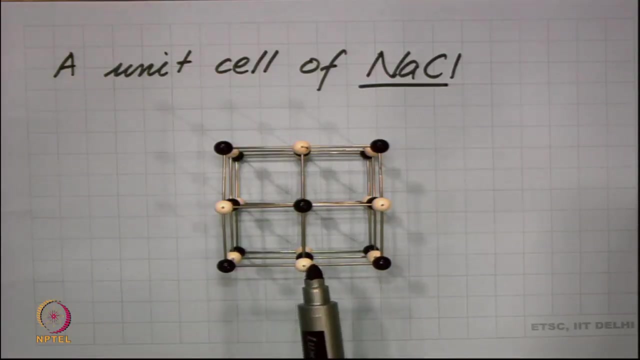 periodic arrangement that these chlorine and sodium atoms are repeating in each direction at equal distances. So, for example, if we look at along the cube edge, we start with chlorine, then after certain distance I find a sodium and then again chlorine, And if I 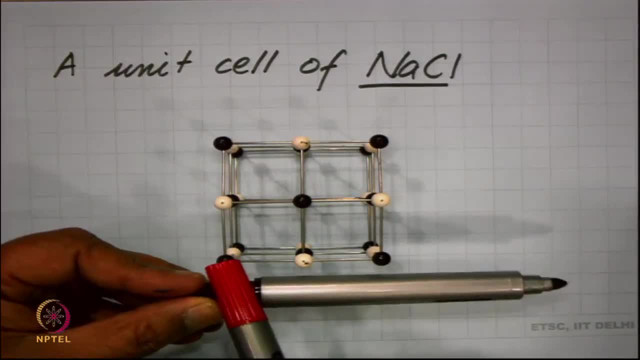 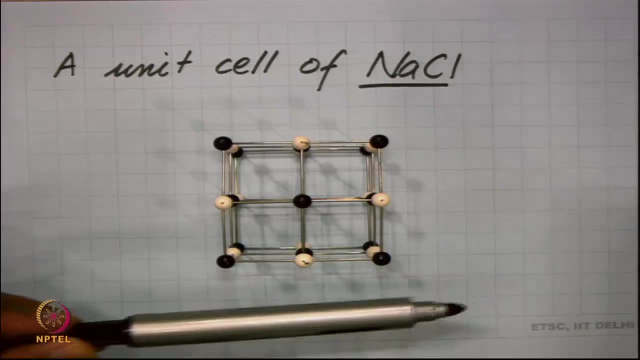 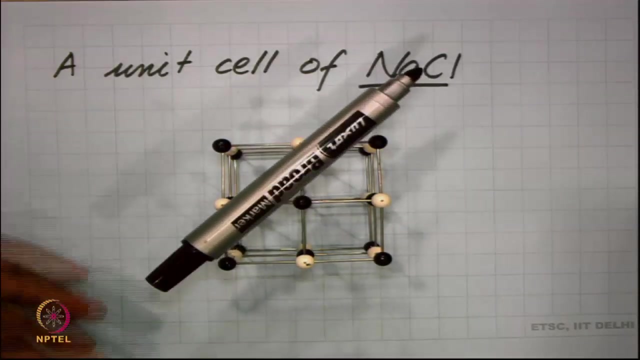 continue in this direction, I will keep finding chlorine and sodium at equal distances. So that is what is meant by periodicity. So in this direction I have periodic arrangement of chlorine and sodium If I go along the phase diagonal. if I go along the phase diagonal. 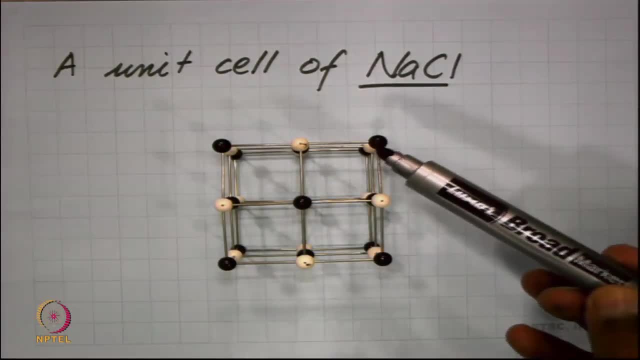 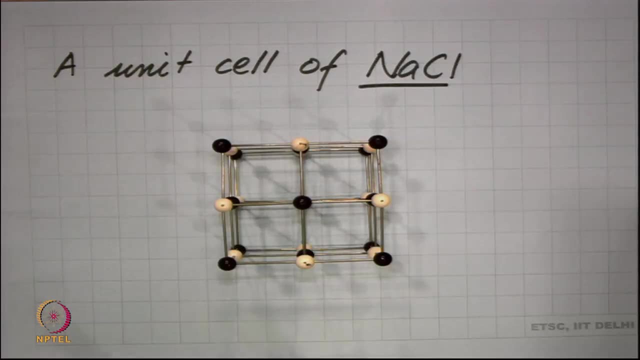 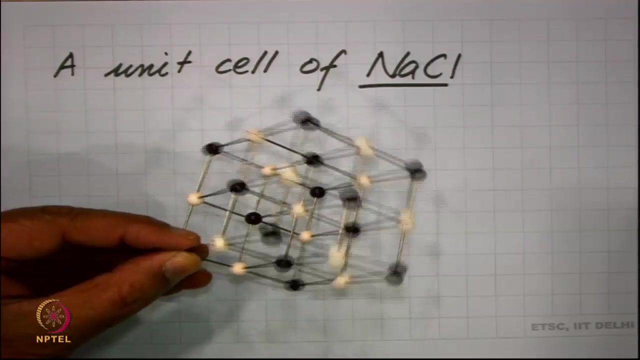 you see we are having chlorine, chlorine, chlorine, Again in this direction. if I continue in the crystal, I will keep finding chlorine at these equal intervals. Same thing is true in all the directions. So I have a three-dimensional periodic arrangement of sodium and chlorine. 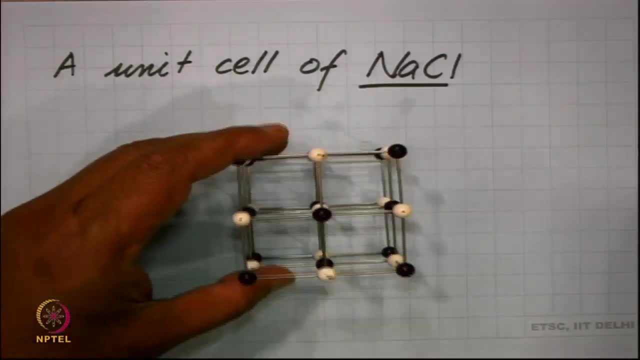 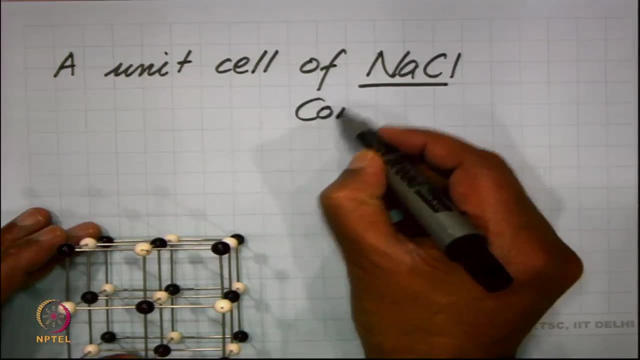 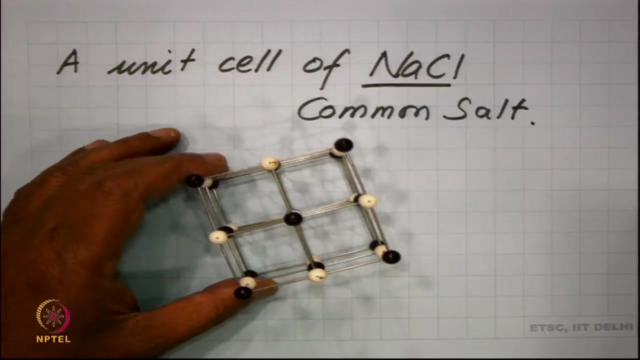 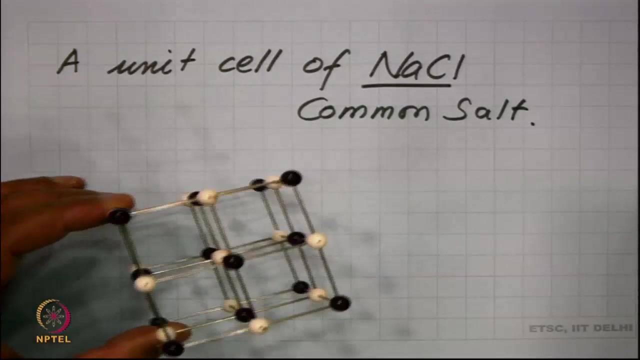 atom represented by this unit cell And this is the crystal of sodium chloride. crystal of sodium chloride, also known as common salt. We will have. we will look at this unit cell and this crystal structure in more detail as we go along At moment. I am showing you just as an example, to begin with. 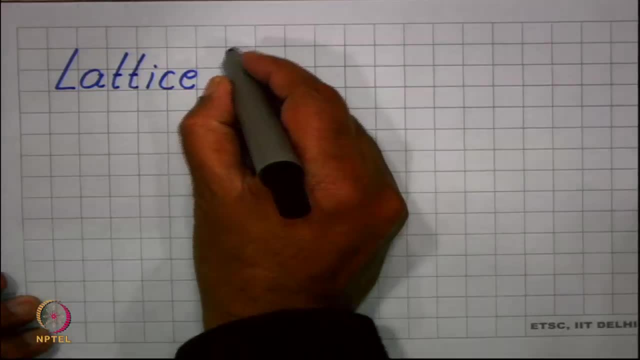 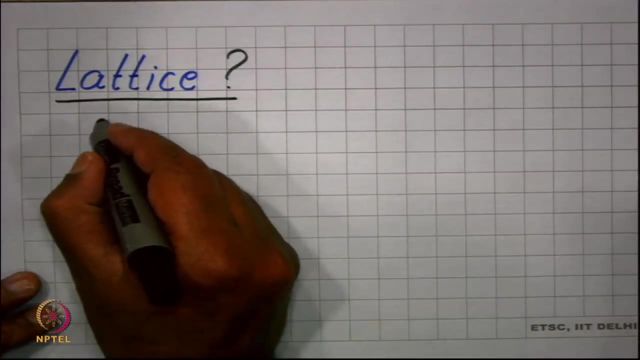 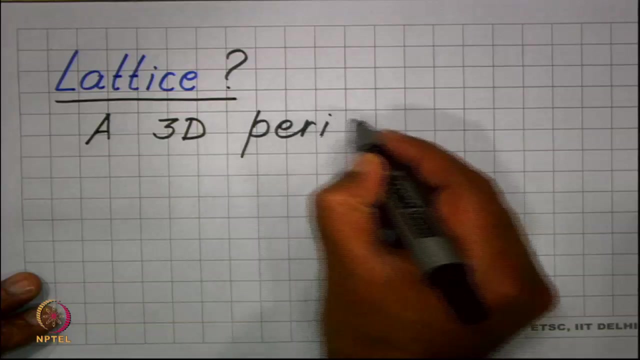 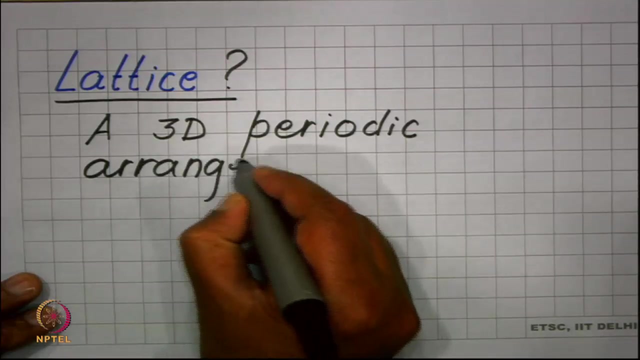 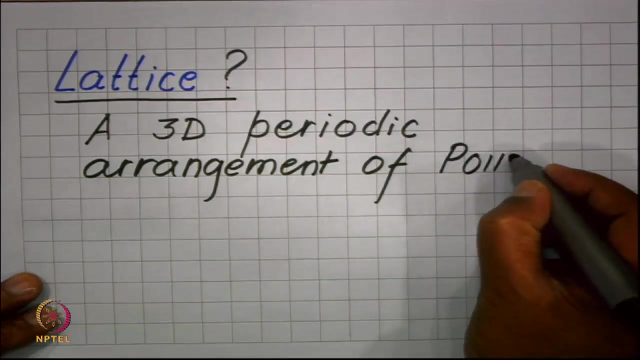 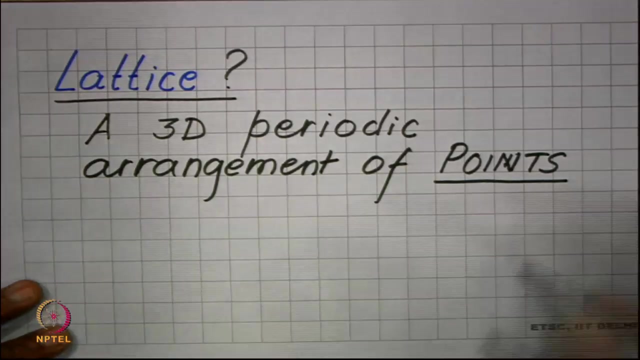 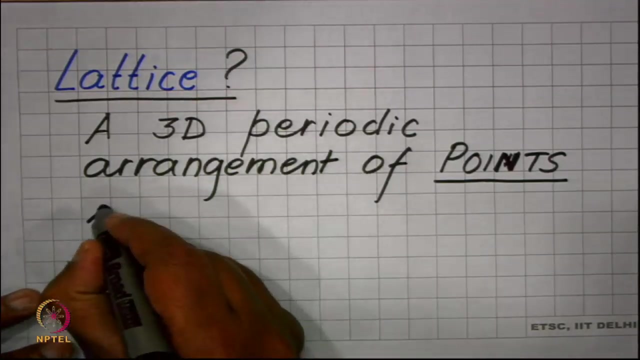 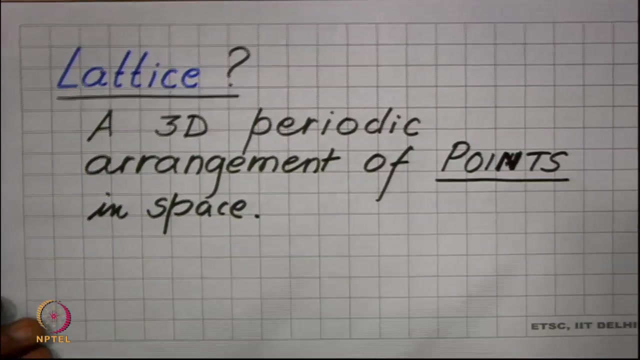 Now I come to the related concept of lattice. what is a lattice and how is it different from crystal? So a lattice is a three-dimensional periodic arrangement of points. Okay, Okay, Three-dimensional periodic arrangement of points in a space. So the difference between: 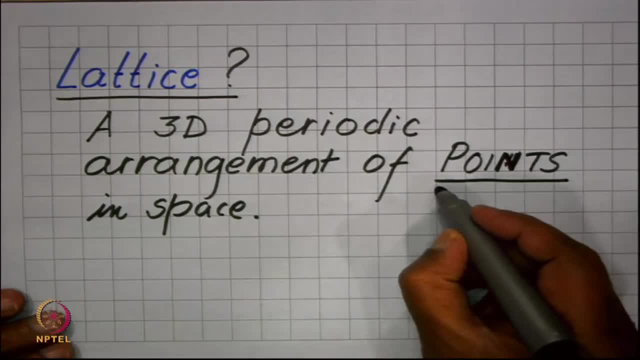 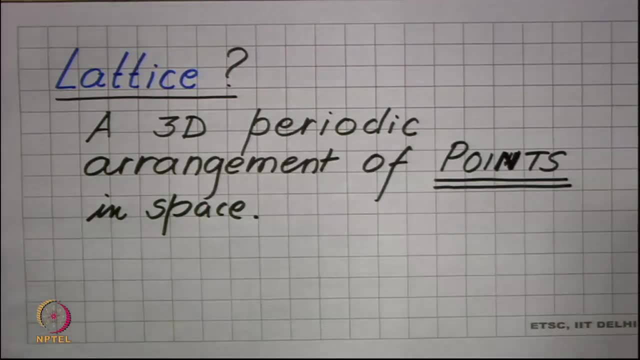 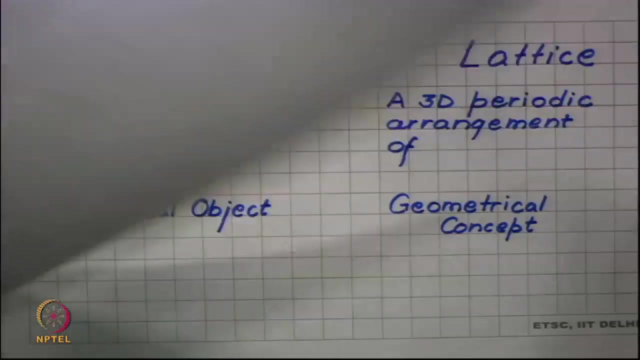 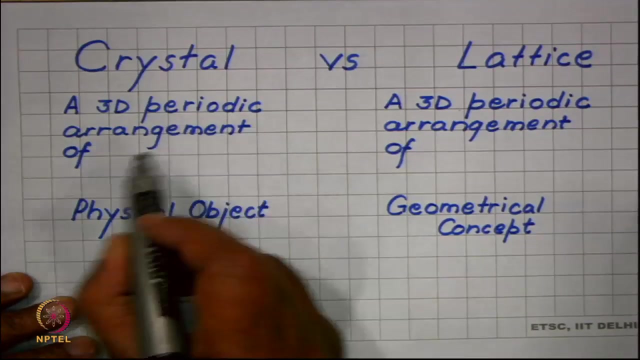 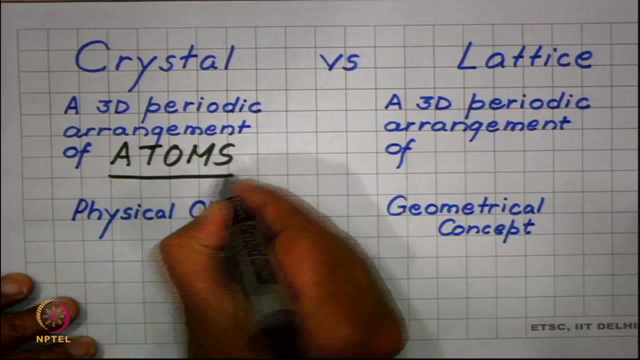 crystal and lattice is whether the points are being considered or atoms are being considered. otherwise, both are periodic arrangement, three-dimensional periodic arrangement. This is the reason for confusion between these two concepts. So let us put that together: Crystal, we said a three-dimensional periodic arrangement of atoms. Let me write that here. 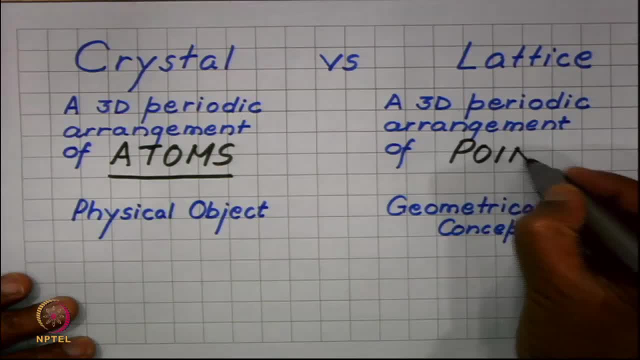 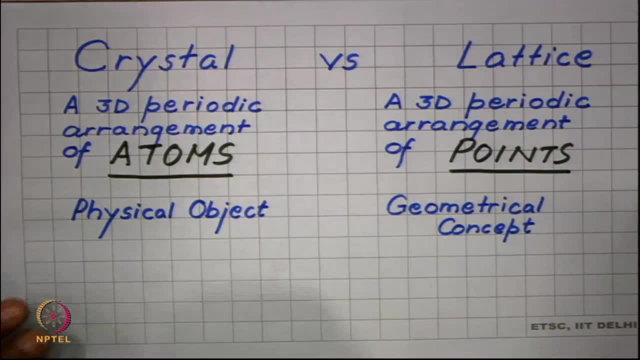 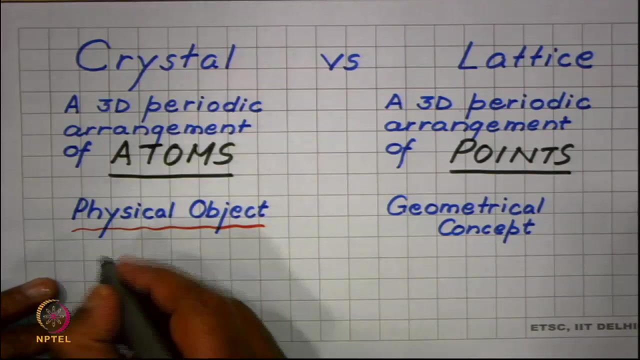 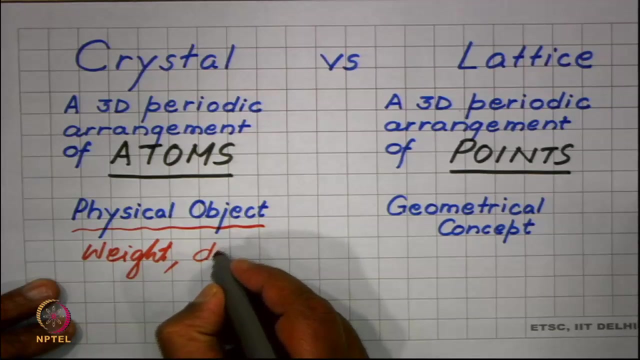 Lattice, a three-dimensional periodic arrangement of points. So you can see, a crystal will be a physical object. Atom is physical object, So a crystal will be a physical object. It will have physical properties like weight- You can weigh a crystal. It will have density- You can measure its. 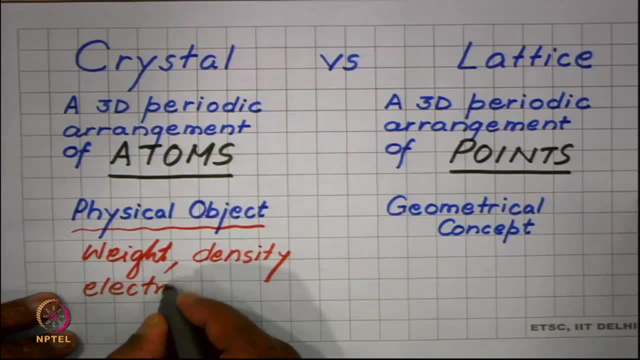 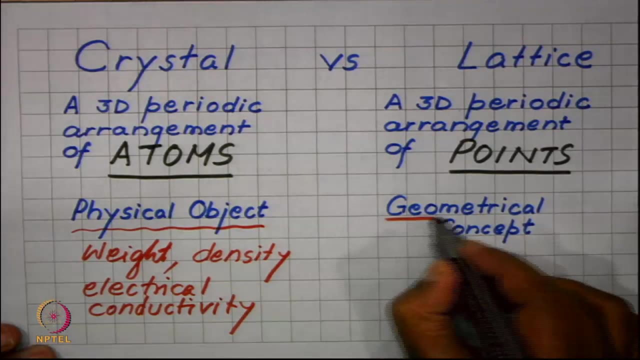 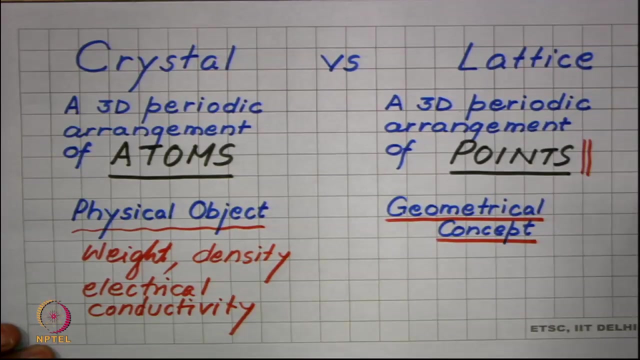 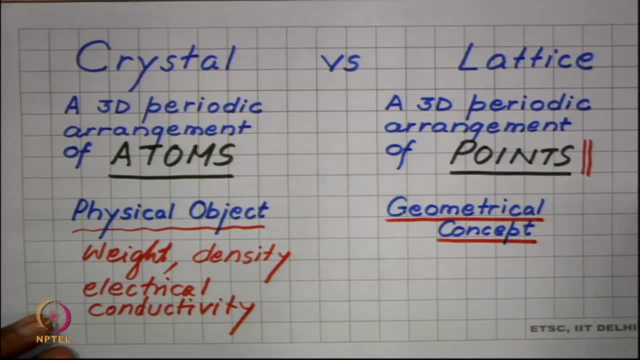 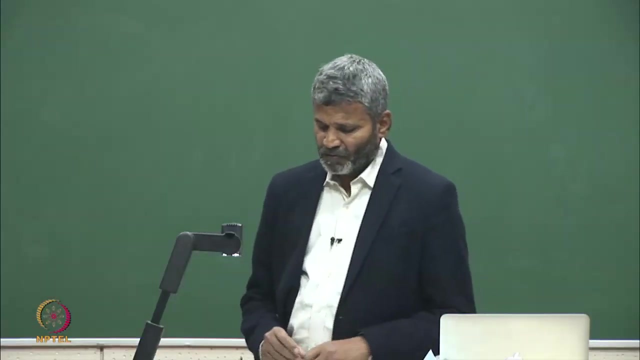 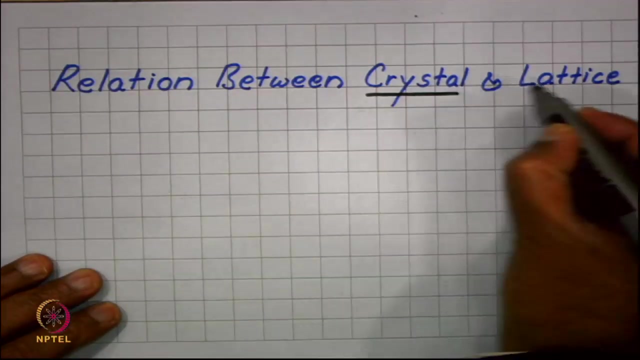 a lattice, You cannot find its density or electrical conductivity and so on, So it has a geometrical concept. We will have only, Ok, geometrical properties. We will make the distinction clear in more detail as we go along. Now, what is the relationship between the crystal and lattice? Both are 3 dimensional. 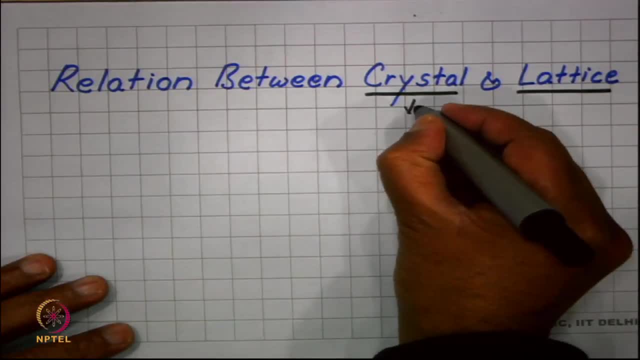 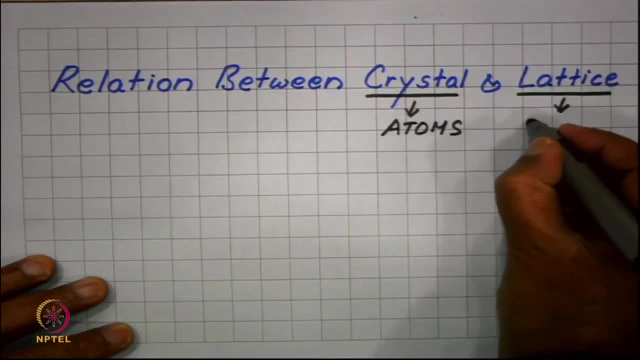 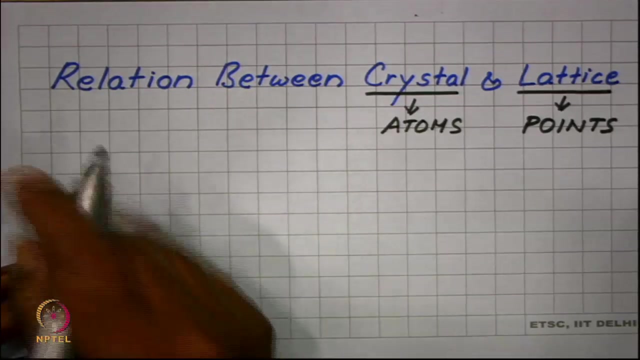 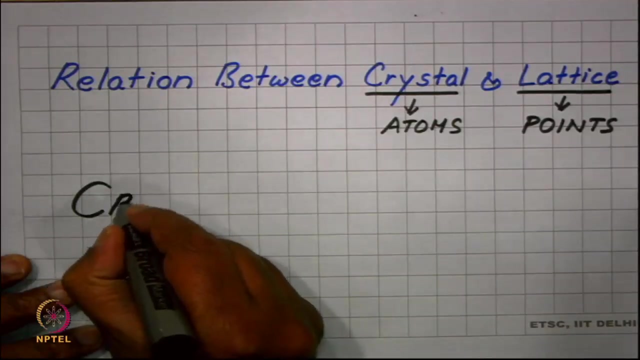 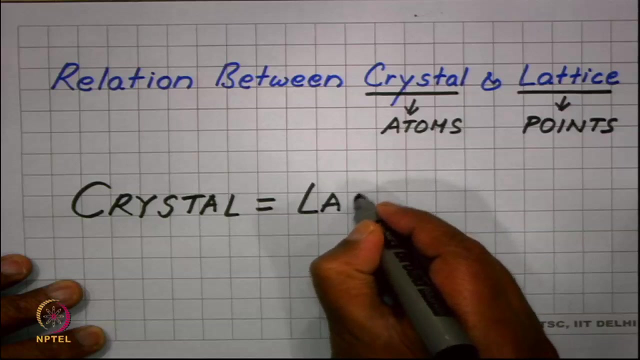 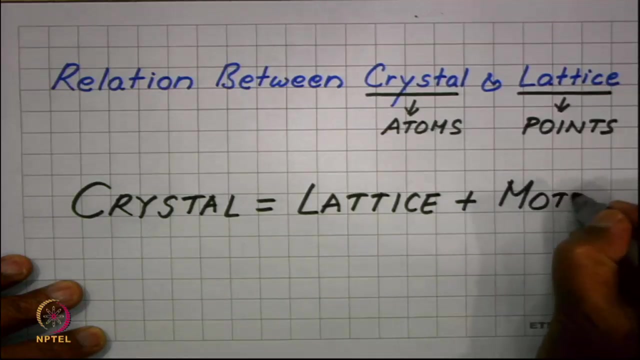 periodic arrangement and we said crystal is a 3D arrangement of atoms and lattice is 3D arrangement of points. So the relationship between them is expressed by an equation: crystal is equal to lattice plus motive or basis. these are synonyms. So 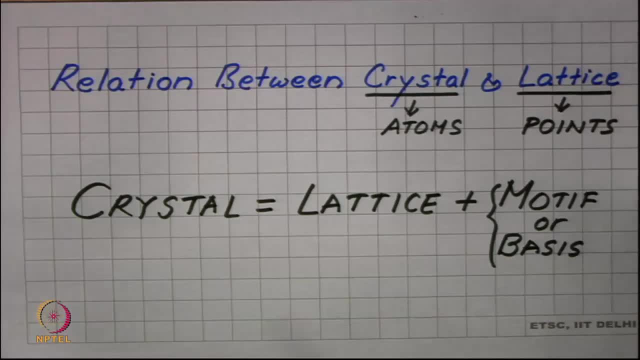 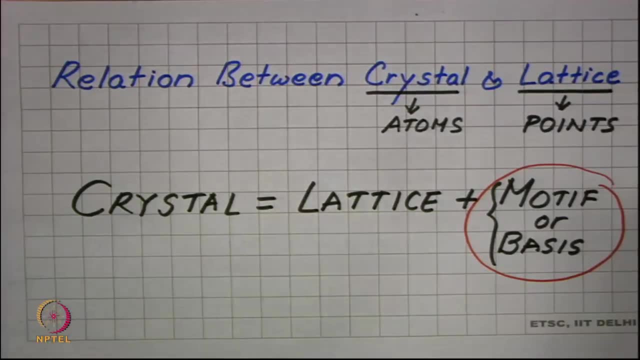 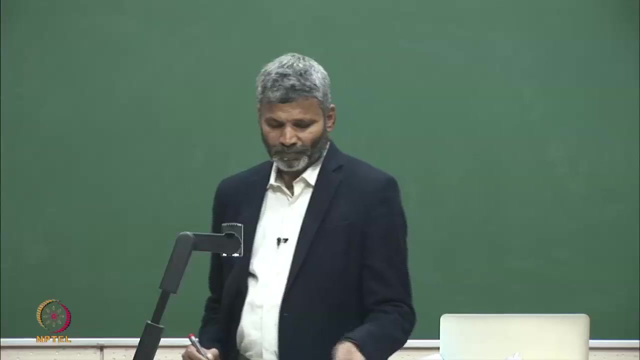 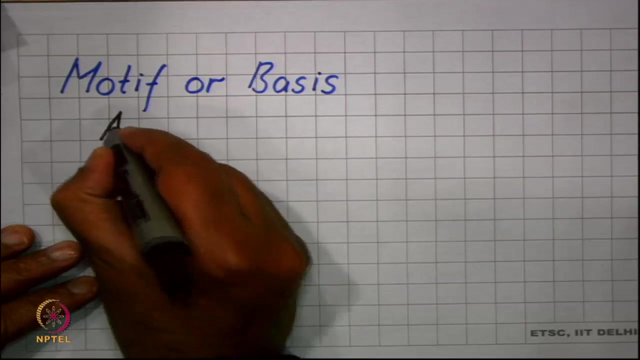 you can call it motive or basis. so this is the new concept we have now introduced. So the linking bridge between crystal and lattice is a motive. So what is a motive is our next topic. So let us define motive or a basis. 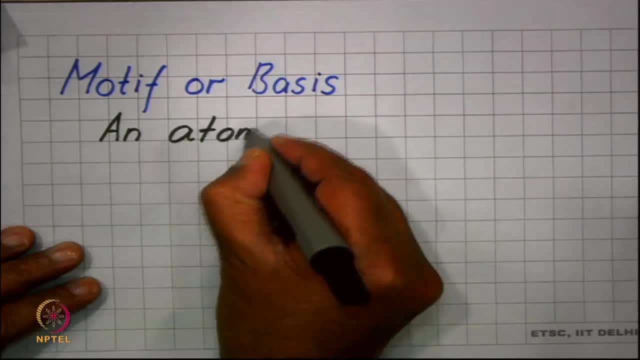 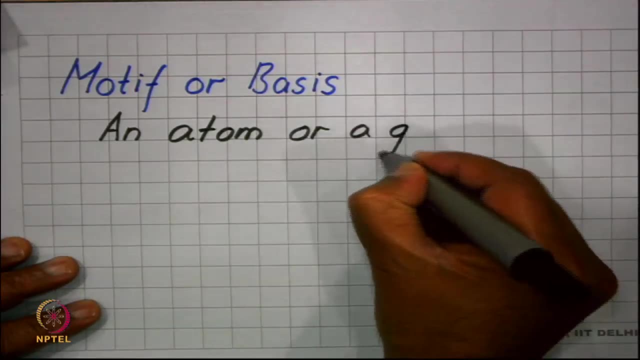 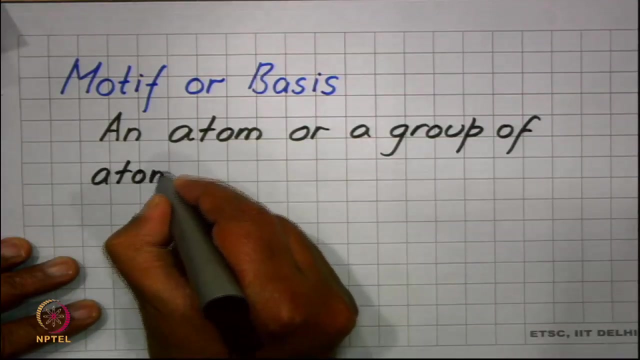 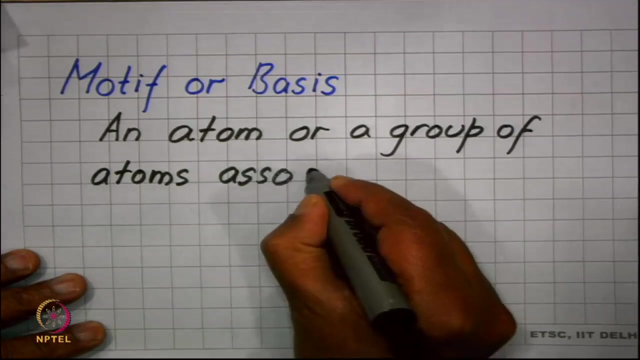 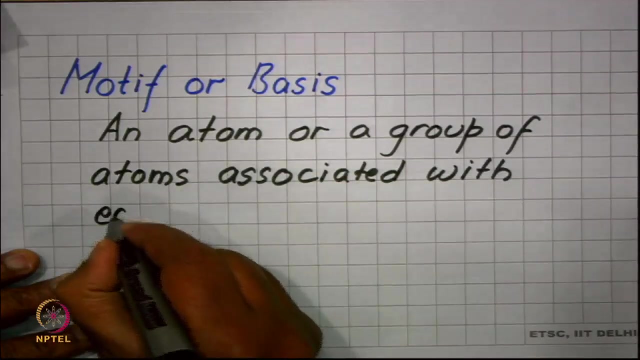 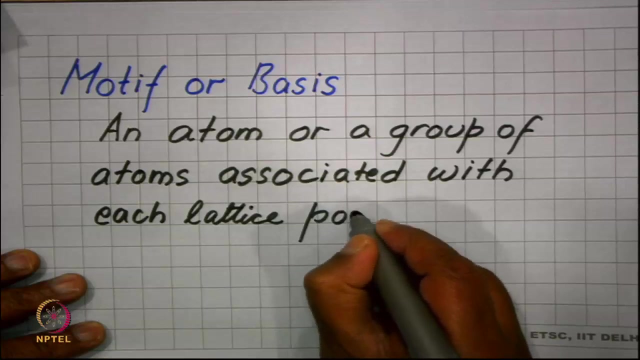 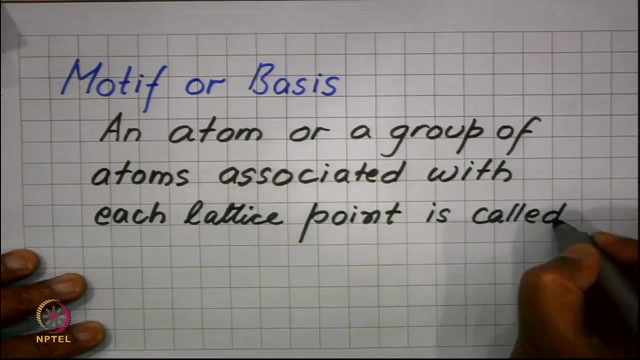 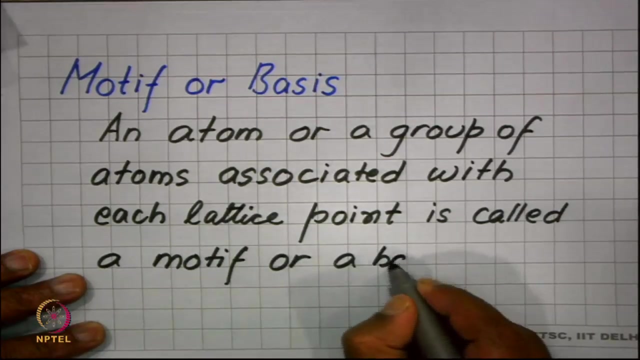 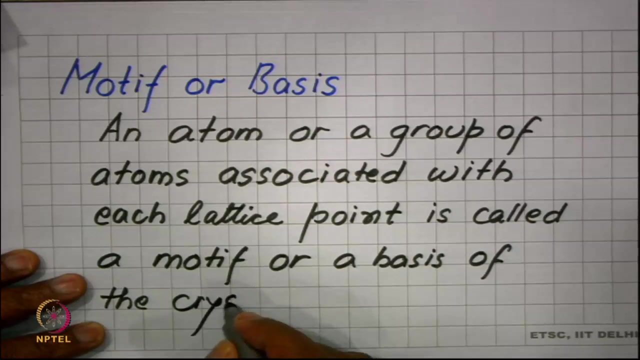 We will define it like an atom For gold and iron. Sometimes a motif can be a single atom or a group of atoms. so an atom or a group of atoms associated with each lattice point is called a motif Or a basis of the crystal. so every crystal had from our equation. if you see, crystal is 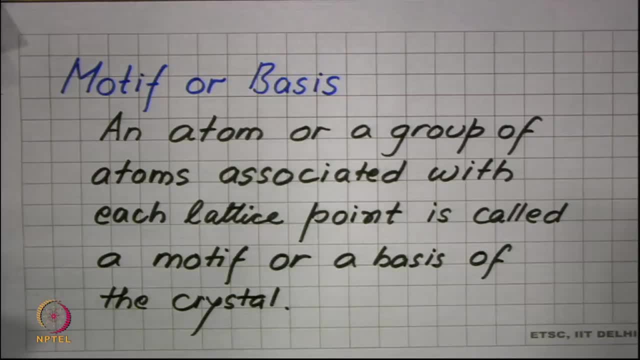 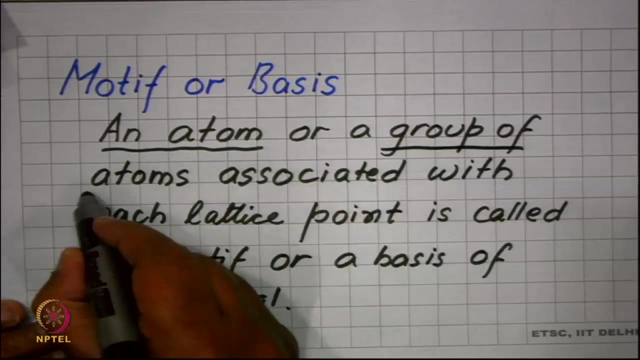 equal to lattice plus motif. so every crystal has a lattice and it has a motif. Lattice is only the periodic arrangement of points. The motif gives you The atom which is being repeated, or a group of atoms. Let us make that distinction more clear. 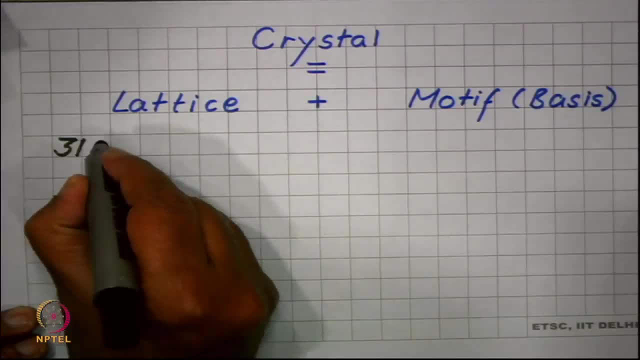 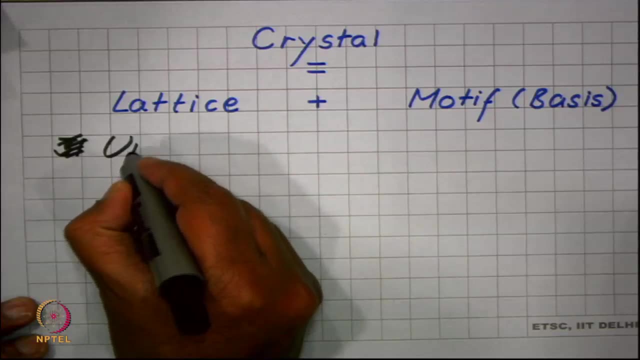 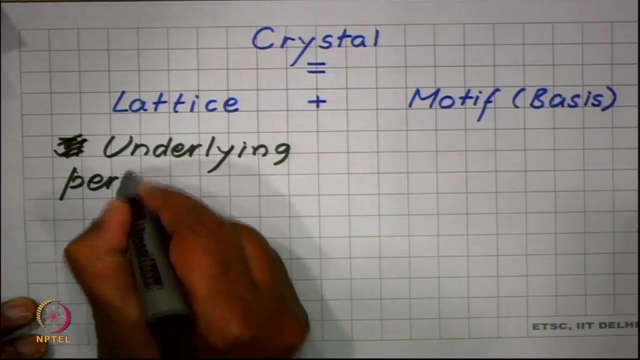 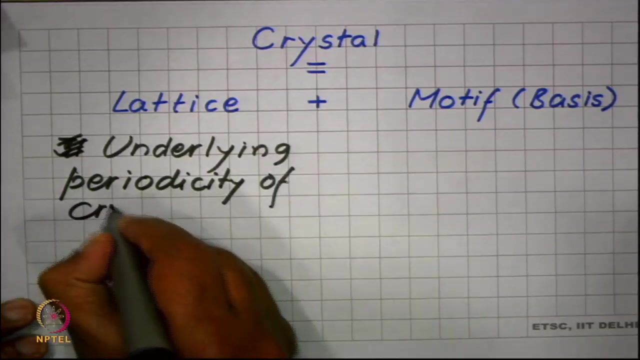 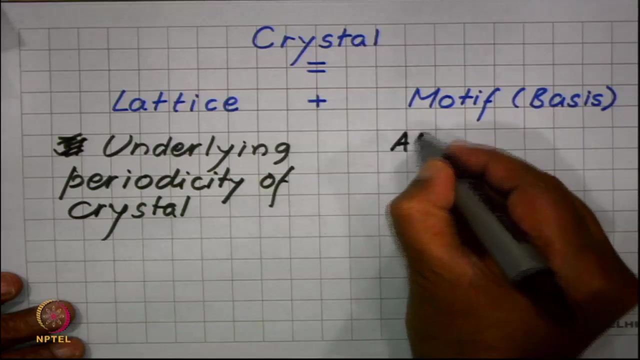 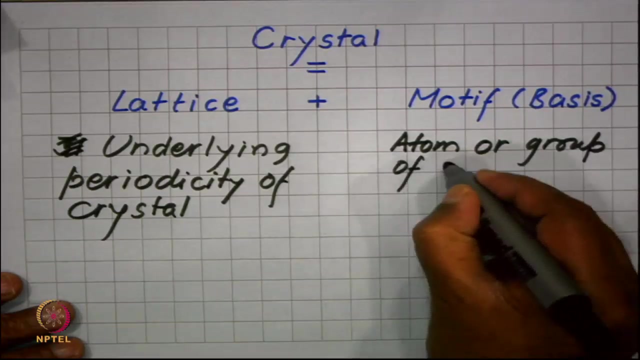 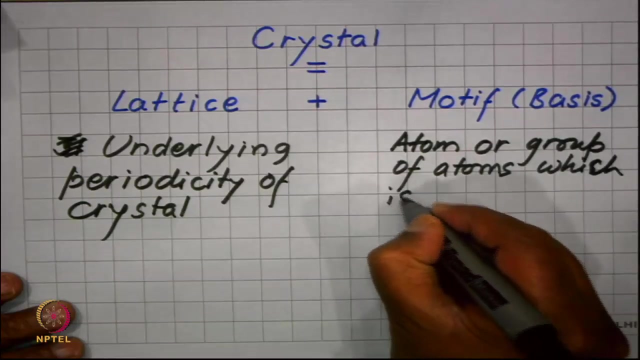 So again, lattice is a lattice- will tell you the periodic arrangement, So the underlying periodicity. so lattice gives you Underlying periodicity of crystal motif, gives you atom or group of atom, which gives you Lattice, Lattice. 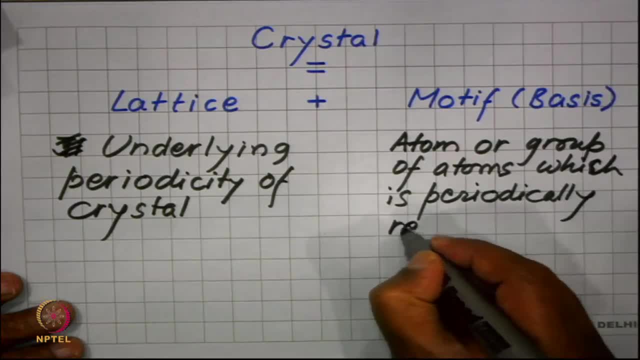 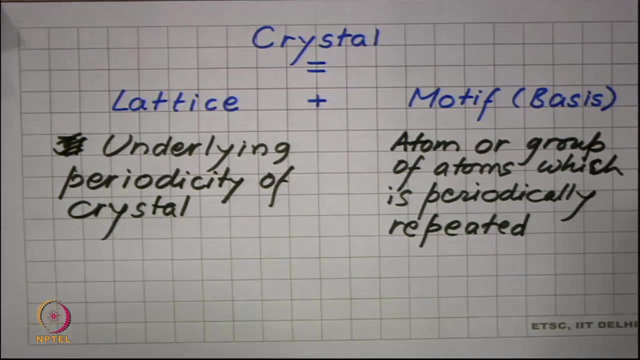 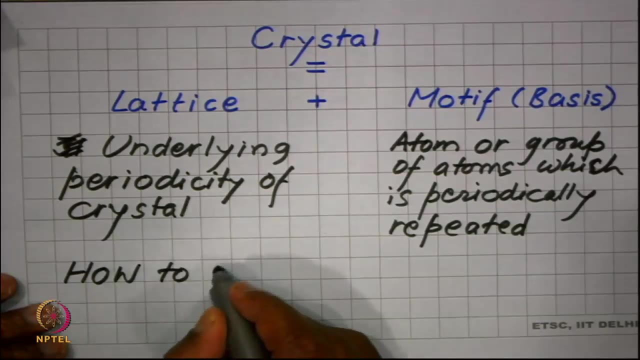 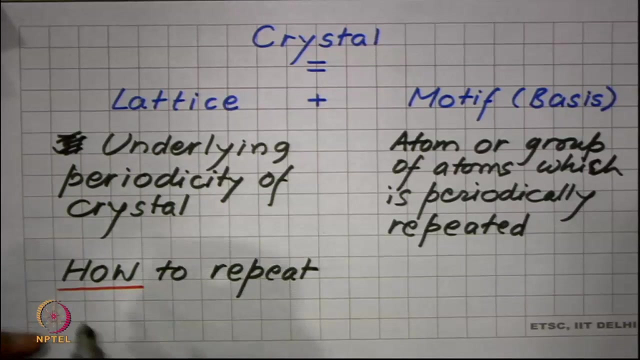 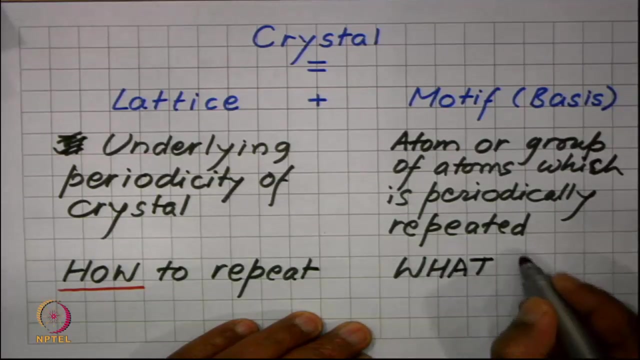 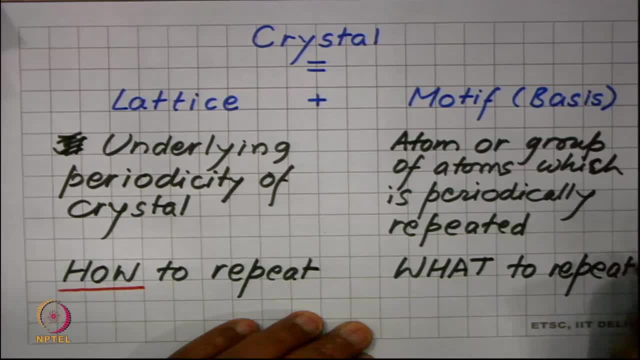 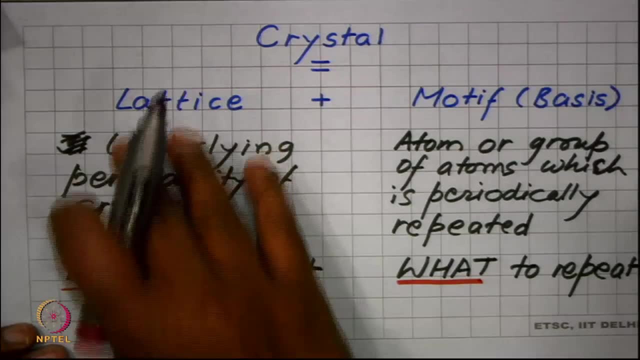 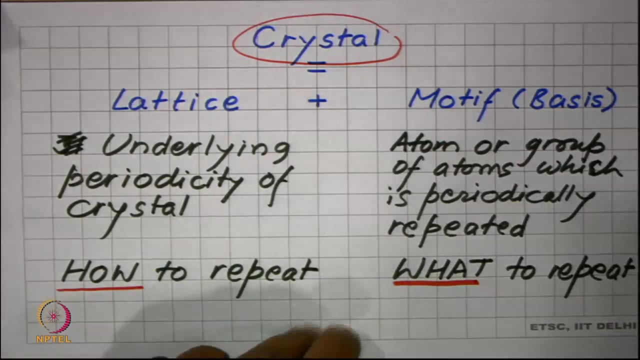 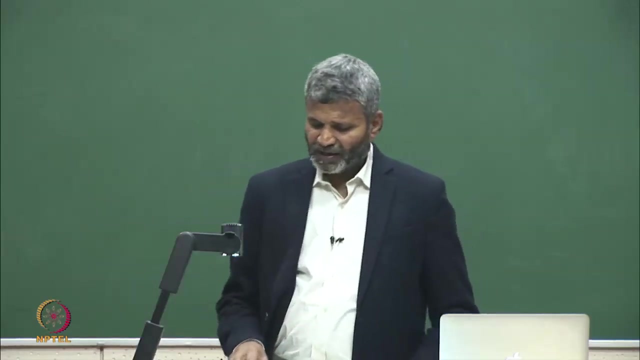 So when you have both this information- how to repeat the lattice and what to repeat the motif- you get the information of the crystal, complete information of the crystal. So let us look at a little bit more concrete example. I have already shown you a three. 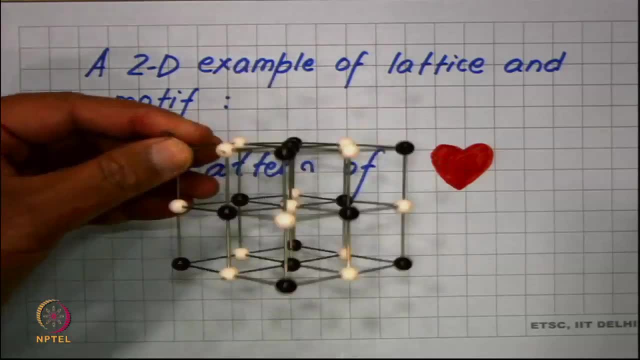 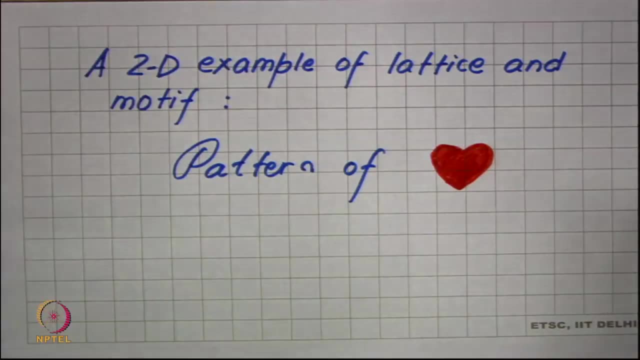 dimensional model of the sodium chloride crystal, but it is at the moment little bit more complicated to analyze, So we will take a much simpler two dimensional example of pattern of hearts. it is an interesting to see a pattern of hearts, so we come here and look at this pattern of hearts. 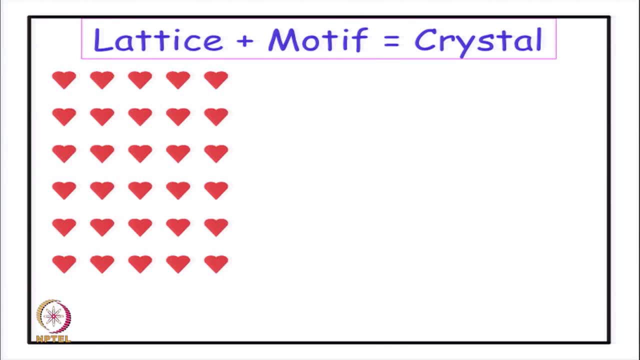 So you can see, what we are doing here is repeating the hearts periodically in two dimensional. so horizontally hearts are coming at equal distance. vertically also they are going at equal distance. So we finally end up with a two dimensional periodic pattern of heart. I want to analyze. 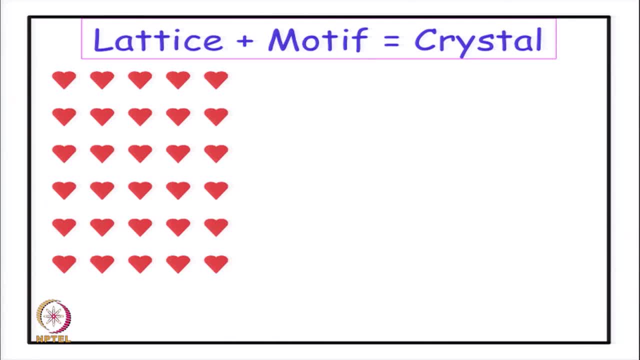 so this periodic pattern of heart, it is something like our crystal, where atoms are repeated. instead of atoms we are now having hearts which are repeating. So this represents. So this represents our crystal, or a pattern. now, if I want to analyze it, this pattern as 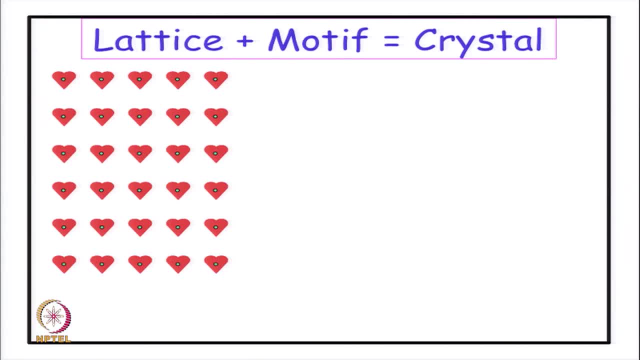 lattice and motif. just like crystal, crystal is a periodic pattern of atoms. now we have a periodic pattern of hearts. this also can be analyzed as lattice plus motif. So first let us look at the lattice. so I have now placed a dot in the center of each. 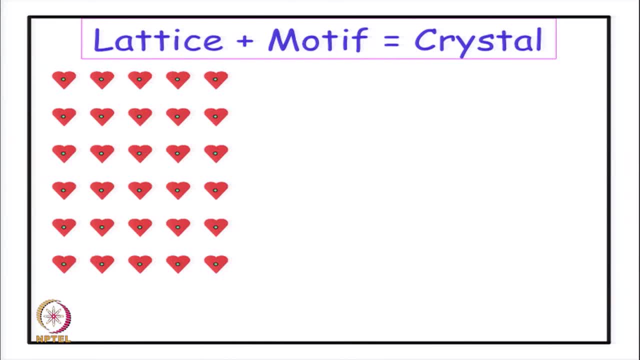 of the heart. so these dots now represent the lattice of this pattern. so if I remove the heart and only leave these points, this gives me the lattice of the heart pattern. but this is not the pattern you can see. but this is associated with the pattern and this: